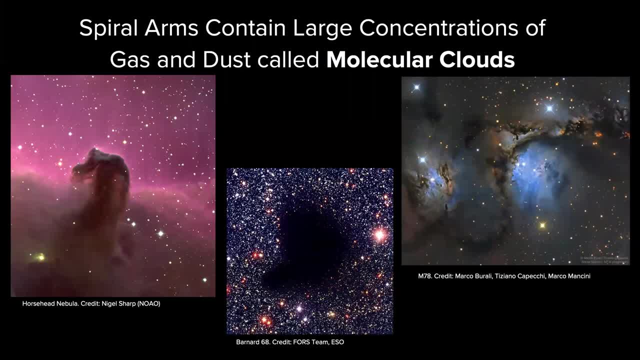 This is important because spiral arms contain large concentrations of gas and dust we call molecular clouds. Molecular clouds can come in a large range of shapes and sizes. They can contain anywhere from a few to a few million solar masses of material and can span sizes from tens to hundreds of light years across. 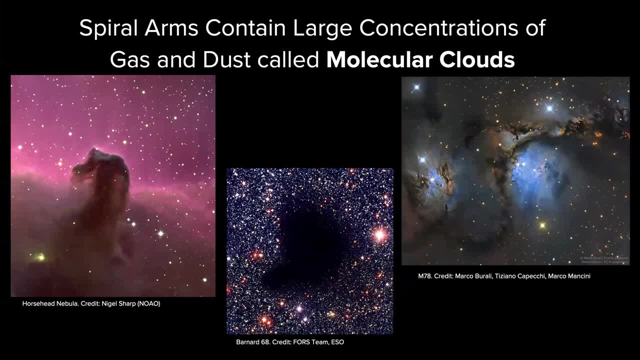 Molecular clouds can appear cool and dark, like Barnard 68, which is shown here in the center of the slide, or they can serve as the birthplace of new stars which heat up and light up the clouds to produce beautiful nebulae, For example the Horsehead Nebula to the left or M78 to the right. 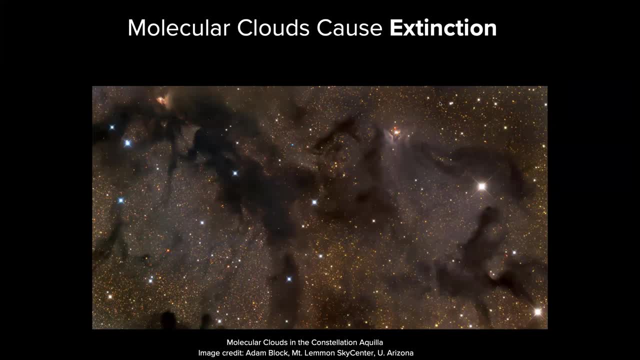 Molecular clouds block the light from background stars from reaching our telescopes, causing them to appear much dimmer than they would otherwise. We call this dimming effect extinction. You can see the effect of extinction in this image of a molecular cloud In the constellation Aquila. the dark regions only appear dark because the 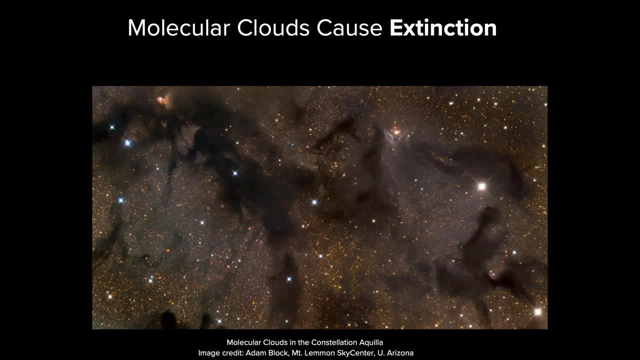 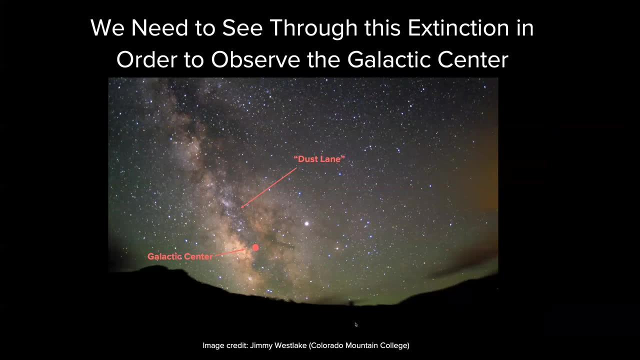 molecular cloud is blocking the light from the background stars from reaching the Earth. So when we observe the galactic center, we need to see through all of this extinction. In fact, you can see the impact of extinction with your own eyes If you look toward the galactic. 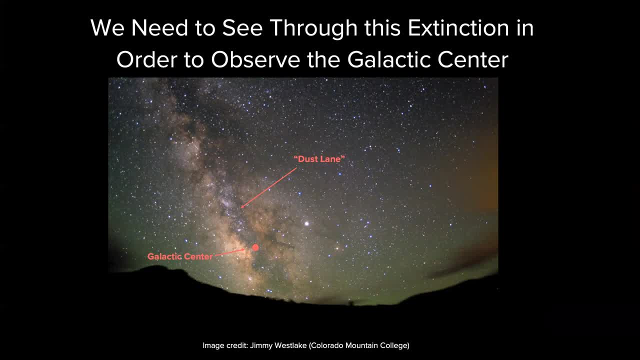 center. on a dark night, you'll notice that the Milky Way looks like a faint stream of light with a giant dark shadow. The faint stream is composed of the light from billions of stars of the galaxy blurring together. This is the pancake that makes up the majority of the galaxy, The dark streak, which is sometimes 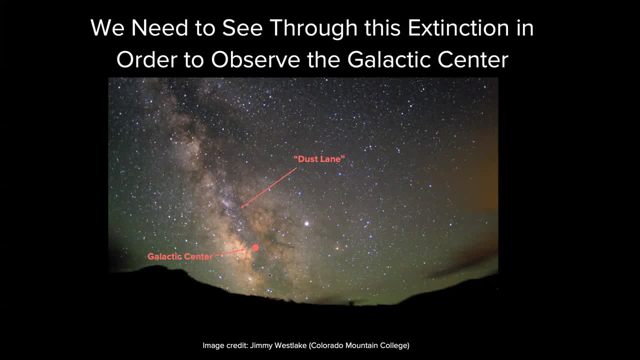 called the dust lane, contains the molecular clouds that block the light from the stars behind them from reaching the Earth. That is why this region appears dark and you'll notice the galactic center is right along the dust lane. In fact, there is so much extinction between us and the galactic center. 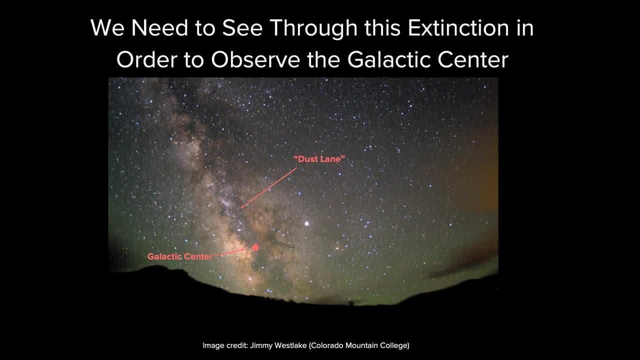 that in optical light- that is, light we can see with our eyes- stars appear 600 times fainter than they would otherwise. This makes the majority of stars at the galactic center too faint to observe even with the most powerful telescopes in the world. So how can we see the galactic center? 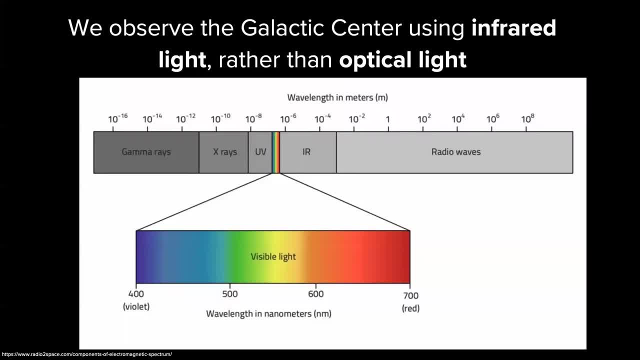 at all. Well, we use a trick: Instead of observing the galactic center in optical light, we observe it in infrared light. So it turns out that objects can emit light across a wide range of energies, which is what we call the electromagnetic spectrum. Here is a diagram of the electromagnetic